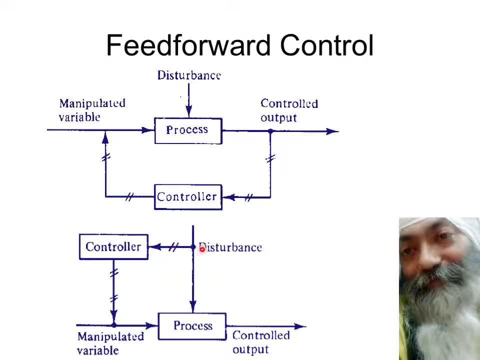 is that this disturbance is measured. This disturbance is measured. Here, you see, there was no disturbance measurement being done. It means that feed forward control, as we are going to see, is going to be applicable only on those processes and applications where the disturbances are measurable. Second, not only are the disturbances measurable, but 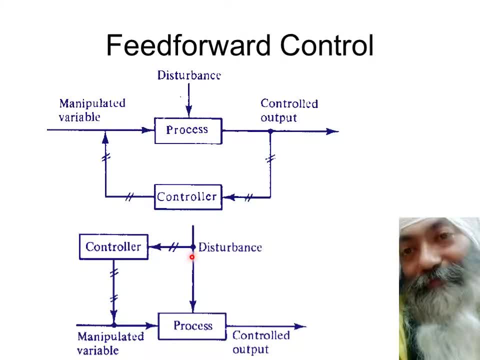 we also know what is going to be the effect of that disturbance On the process and ultimately on the controlled output. we must know that how is this disturbance going to deviate this controller output, whether it is going to increase the controller output and to what extent, or it is going to decrease the controller output and to what extent. 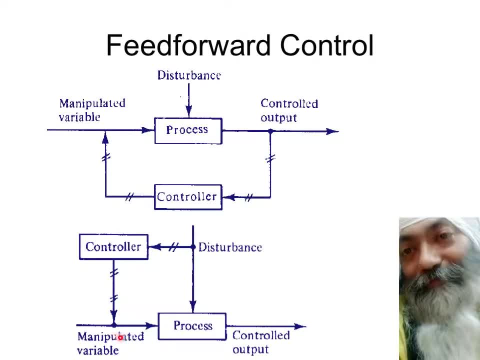 And we also know, we also know the effect of manipulated variable on the same controlled output. If we know that, then measuring the disturbance and then estimating what its effect is going to be on the controlled output, we decide. we means the controller. it decides to have exactly equal and opposite effect of the change. 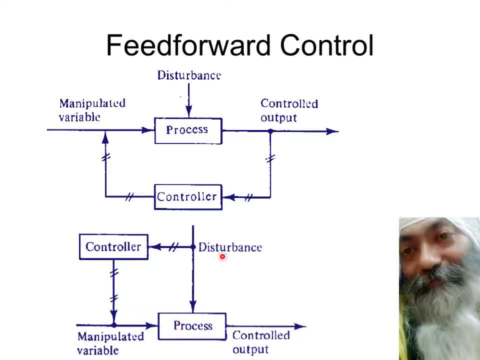 in manipulated variable, So that whatsoever was the likely likely effect of disturbance on the controlled output, we will introduce exactly equal disturbance on the controlled output and opposite effect of manipulated variable on the same controlled output, so that the effect of disturbance on the controlled output and the effect of 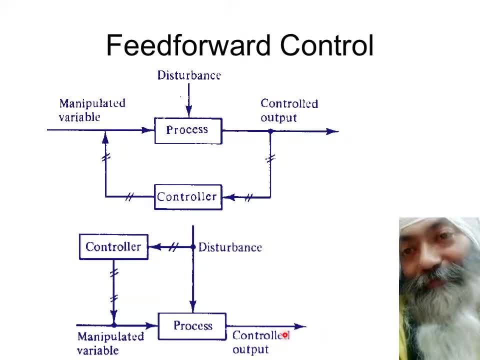 manipulated on the controlled output. they cancel each other and the controlled output remains at the same point, remains at the same point, so its action is taken before the controlled output starts changing before, and that's why it is called feed-forward control. the upper one is feedback, the lower one is 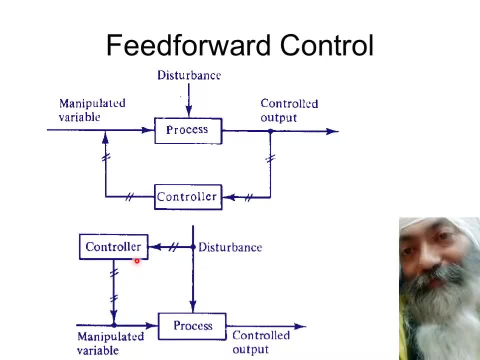 feed-forward. so the two things which we see is that first of all, the disturbances have to be measurable and second thing is that the effect of disturbance on the process and the effect of manipulated variables in the process that should be exactly known to us means the model of the process should. 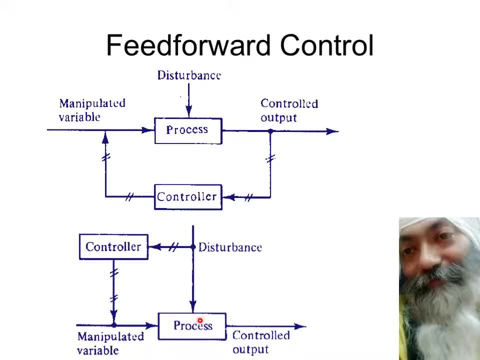 be easy to follow, because the intent of the method is that the ammo is collected be known to us exactly. only then can we design the controller to have this feed forward effect. and the good point, the advantage of this, is that the control output never, ever gets disturbed. 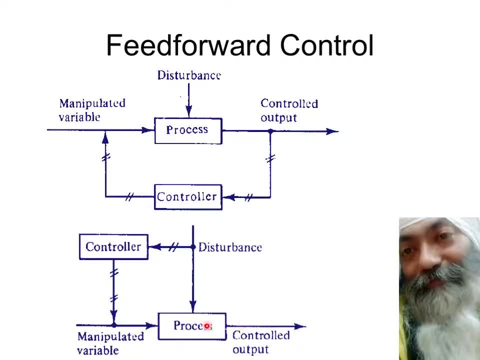 we don't take action after the damage is done. we control the damage before it is done and the output remains at the same point as it was, without any deviation. so this is a feed forward control, with its own advantages and disadvantages, as you can see. we shall be studying this. 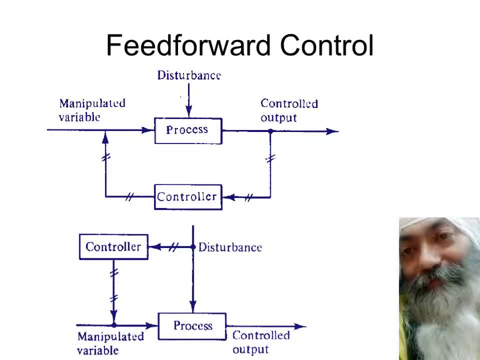 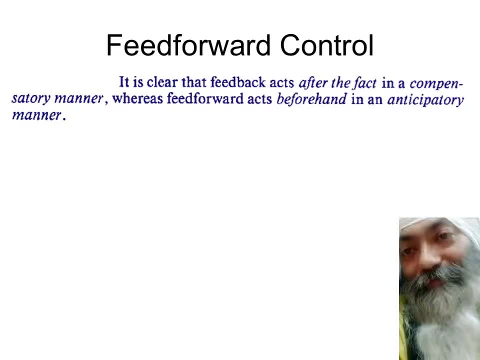 for a while in the next slide as such. so, my dear friends, it's clear that, if i'm allowed to read it, verbatim feedback acts after the fact, in a compensatory manner, whereas feed forward acts beforehand and in an anticipatory manner, and this we will see in the next slide. 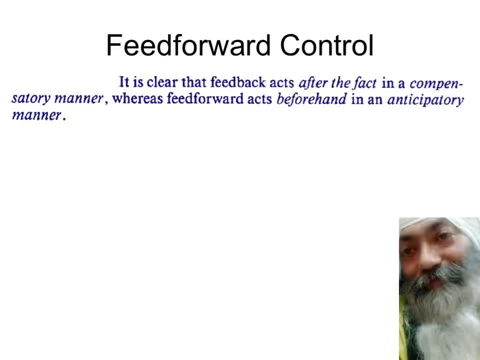 you shall be again explicitly explaining with the help of a steam boiler. just have a look at what's this steam boiler doing. this steam boiler is getting the feedback, is getting the feed water. it's getting the feed water, it's entering into the drum, it's being heated, it's converted into. 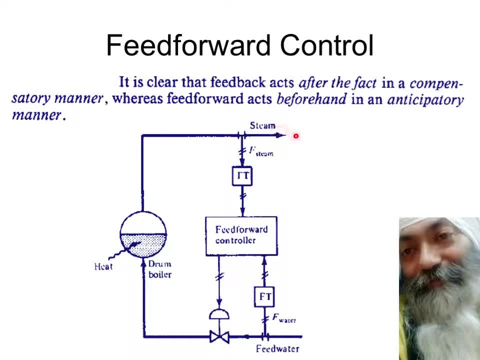 steam, in very simple terms, and the steam is being given to the plant. now the plant, it has its own requirement of the steam. it can extract more stream, it can stop the steam altogether, and so on and so forth. so these changes in the steam outlet are disturbances. these are disturbances, suppose. 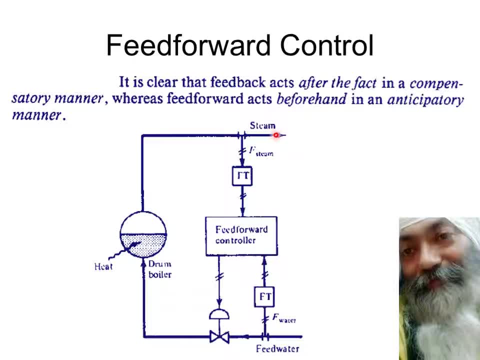 the steam extracted from this boiler. it suddenly increases. someone opens the wall of steam in the plant and the flow rate suddenly increases. now the steam boiler is getting the feedback, is getting the feed water. now this increase in the outlet of steam is going to have its effect on the 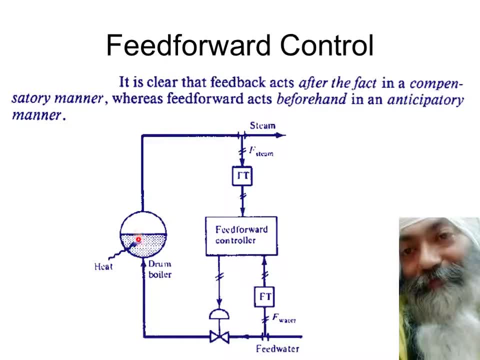 level of the drum and the level will start falling. level will start falling. we are not measuring the level, we are not taking the feedback from the level of this drum. what we are doing is the disturbance is the outflow of the steam, and we measured the disturbance itself. this is a flow transmitter, FT, and this is given to the. 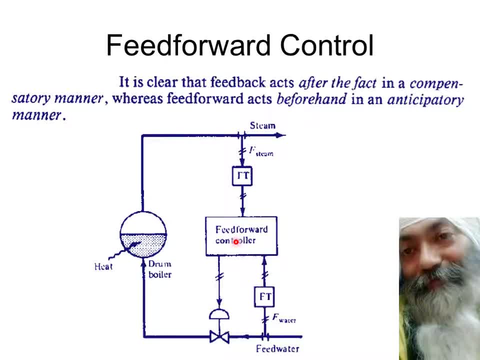 feed forward controller and we know in very simple terms the effect of increased outlet of steam on the level which you want to control, without measuring the level. instead, we are measuring the disturbance and what we do is that if the outflow of the steam increases. it's a very, very simple model. 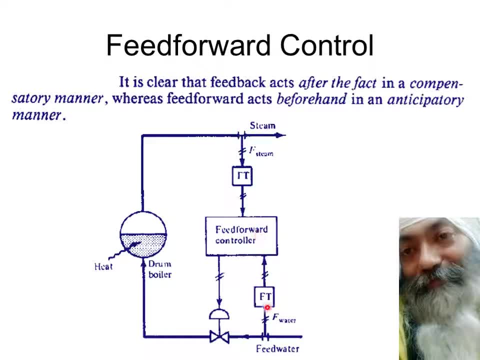 if this has increased by 10%, I will increase the feed water, the inflow of the water, also by 10%. as simple as that. this is a feed forward control, is the simplest kind of feed forward control. that, this ratio, it's a kind of ratio. you. 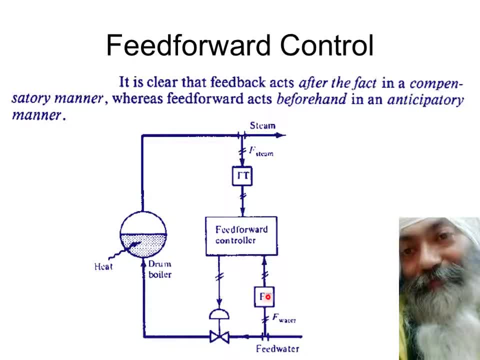 can see. if this increases, then you also increase this. now, the same ratio, 1 is to 1 if it is in terms of mass, not in terms of volume, because you know volume of steam is different from volume of water in terms of mass. you can see now. 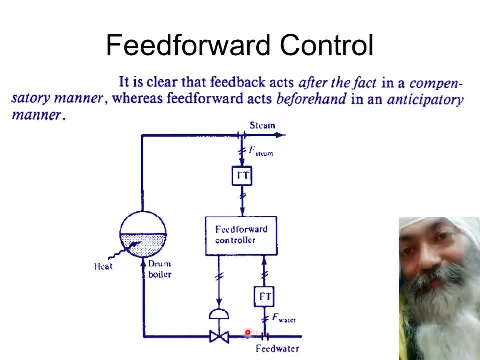 you As you increase the inflow of the feed water using this controller, using this valve. its effect on the level exactly compensates for whatsoever. was the effect of increased steam outflow on the level. Exactly the same will be the effect of increased feed water on the level of the drum, but in the opposite direction, and so this level will remain the same. 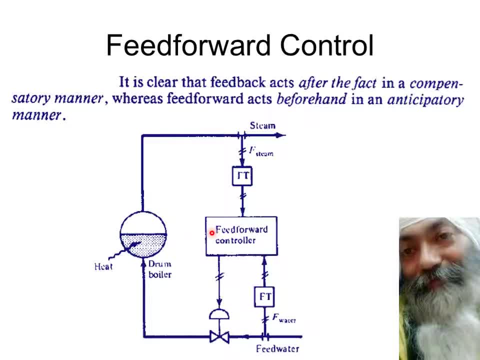 We have made use of feed forward control and not feedback. We are not waiting for the level to come down and then error is calculated and then nothing of that sort happens. This is the simplest example, but we will go in for another example which is more complicated. 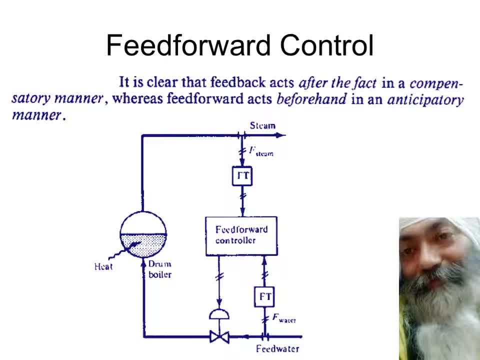 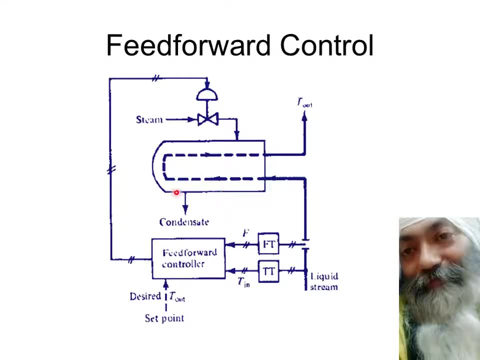 More complicated and more difficult to implement as well. in the next slide. What you see over here is a heat exchanger. Some liquid stream is going in and it's getting heated and you want to increase the temperature and you are able to achieve that temperature. 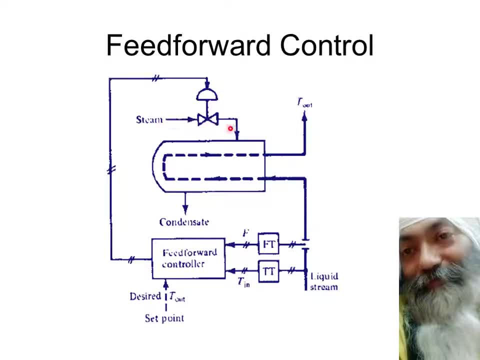 Now some amount of steam is One is flowing to this shell and it's transferring the heat, and the condensate is coming out from this part of the shell. Now this output of the entire thing can have number of disturbances. If the flow rate changes, this temperature will be affected. 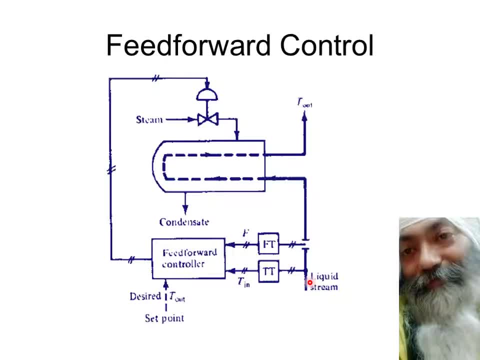 If the temperature of this liquid stream- that also liquid stream that also changes, It becomes higher or less, If the temperature of this liquid stream- that also liquid stream that also changes, It becomes higher or less, then this t output will also change. but we are not taking feedback, we are not measuring. 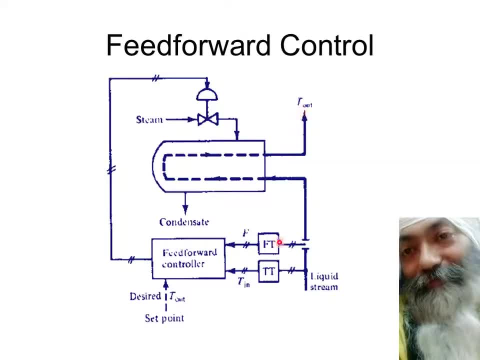 the controlled output, but rather we are measuring the disturbance itself. disturbance can be in the form of change in flow rate, disturbance can be in the form of change in temperature. and these disturbances, they go to the feed forward controller. the feed forward controller has exactly the exact mathematical model of what's going to happen on account of the increased flow rate. 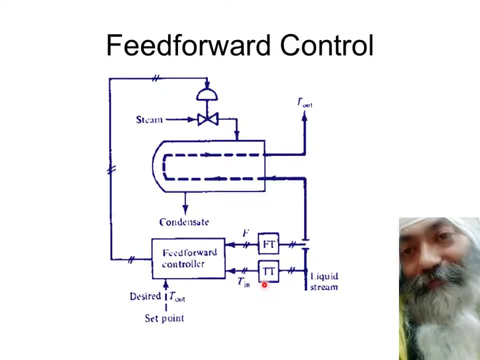 what's going to happen on account of this increase or decrease in temperature and that also knows how to compensate for this, and therefore it will exactly change that much amount of steam which is going to nullify, because effect of this change in steam has to be equal and opposite to. 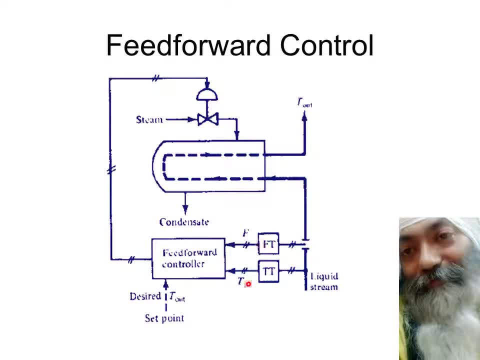 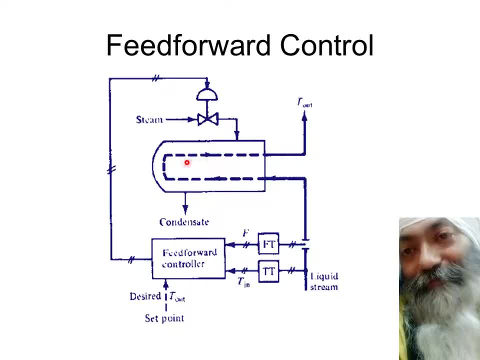 which we required, and we shall be seeing these things in in the subsequent slides also. but here the modeling is much, much difficult. as in case of the boiler, it was very simple that if the flow out rate, mass flow out rate, increases by 10 percent to increase the mass flow rate of 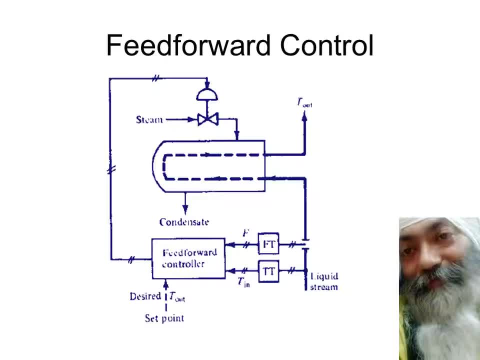 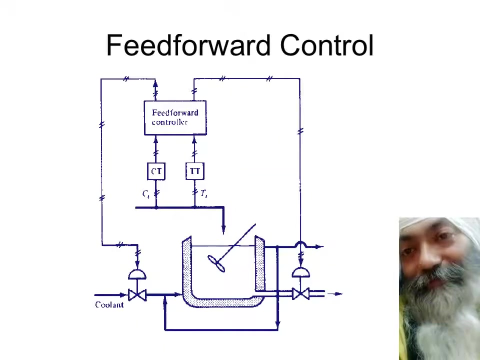 issuing some output, also by 10%. here things are quite complicated and they require a good deal of modeling and good deal of estimation and good deal of prediction of all the things, so that they can be exactly equally and oppositely canceled to make the controlled output remain at the same set point. 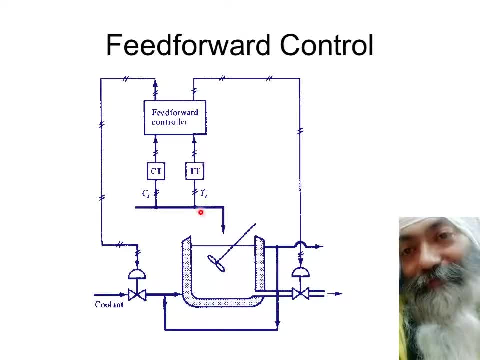 this is the third example and perhaps the last one. one can give you so many examples on that. and again you have what you see is a kind of continuously stirred tank reactor and it's an exothermic reaction taking place. so you want to keep the temperature constant of the entire thing, so you make some 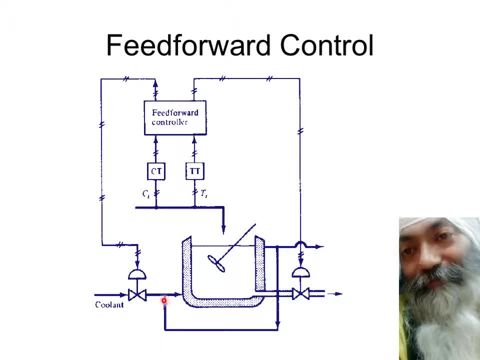 coolant flow through it and the coolant is going in at one point and coming out from another point and what you do is what you do is that the disturbance can be in the composition of the inlet, disturbance can be in the temperature of the inlet, and both are going to change the 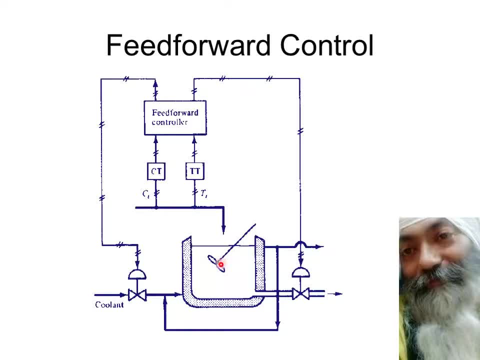 temperature. so instead of waiting for the temperature to change over here and taking the feedback of temperature and then controlling the coolant, what we see is we measured the composition, we measured the temperature. we have the model. we know how it's going to affect the temperature. we also know how the flow is going to change. flow of coolant is going to change the 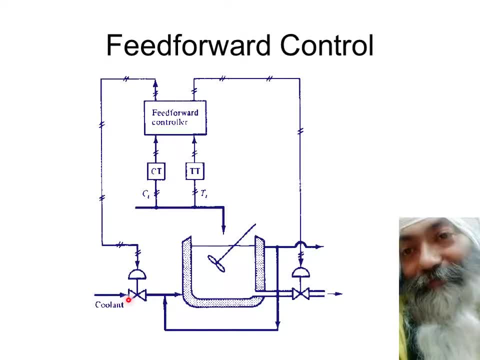 temperature of this and this coolant is changed by measuring the disturbance occurring here or here, or in both of them simultaneously, and then the coolant flow rate is adjusted exactly to the point so that whatsoever is the effect of this disturbance, or this disturbance is cancelled by an equal and opposite effect of flow of coolant. 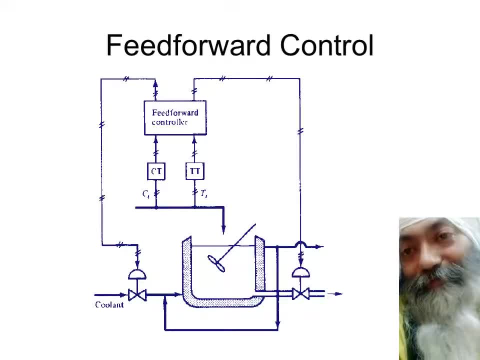 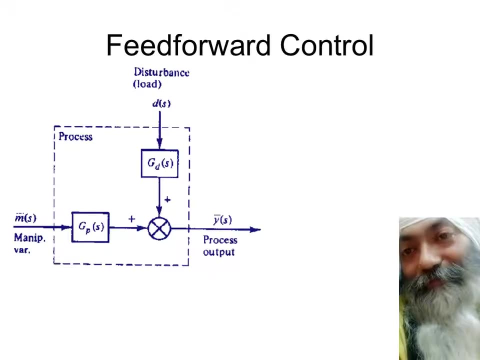 in this direction. so the temperature of this always remains the same. this is one another example of feed forward control. coming to the concept of going its mathematical modeling, as you can see it, simple process, simple process. it has its transfer function as gp: how manipulated variable is going to? 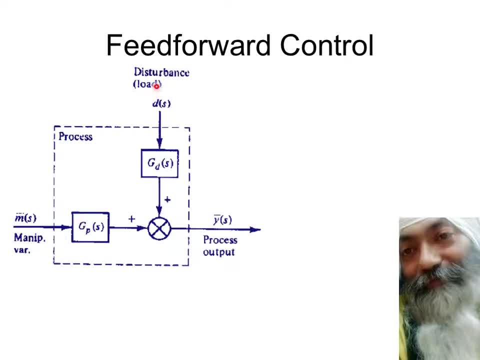 affect the process? is gp? how disturbance is going to affect the process? is gd from here on, how many variable thirsty gps how? on my channel, t was a primary class method of streaming, so basically on a single output of TW, but sent to you to answer these two basic questions. 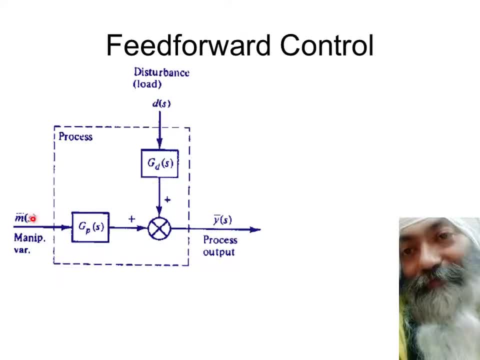 sum of disturbance, as a sum of the mathematical variable. both are together to give the output of the process. so why else? is equal to DS into GDS plus MS into GPS. this is one simple equation, as you can see from here by yes is equal to. we want this ys to be equal to set point. we want output variable to be equal to set point. so i can. 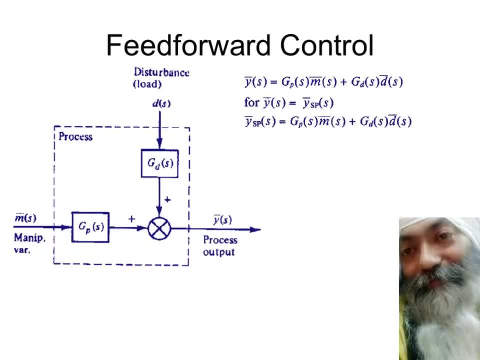 this value of sp in the previous equation and i will get ysp is equal to the same thing. the same equation, as you can see up, is repeated over here and from here i will try to get the value of ms. what will be ms? i will divide the whole equation by gd, so this ysp will be divided by gd. i will. 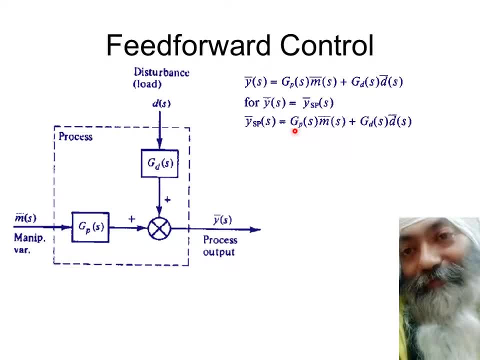 subtract ds from it and then i will divide it by gp to get the value of ms. this is what is going to be done. as you can see, this ms ultimately is equal to ysp divided by gd. everything was divided by gd, so this also comes over here. so, ultimately, what you see is that this is the value of ms. it's. 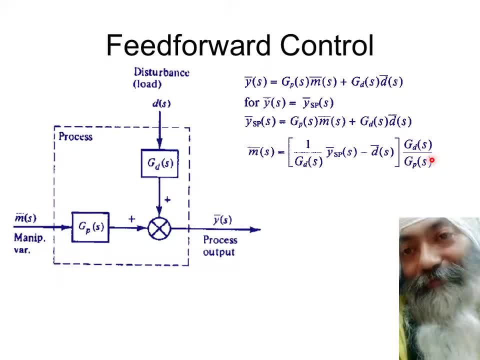 it's manipulated variable comes out to be this thing. now, this thing gd upon gp. is the controller action which is acting on the error which is produced on account of the disturbance or whatsoever? is the change in set point? we change the set point. even then it will be. it has to be multiplied by one. 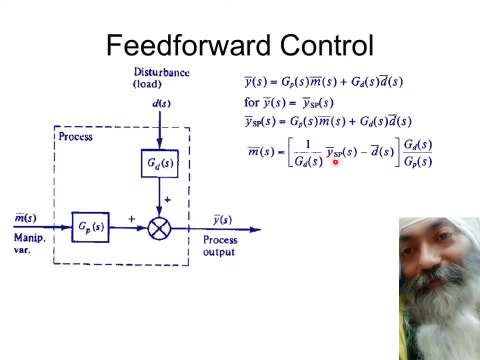 upon gd, that factor we will be controlling over here, or this, this thing, gd upon gp. what is gd? gd is the model of the process, on how the process is going to change as per the disturbance. what is gp? gp is again the model, model of gp over here, as you can see over here. so this thing, we call it as. 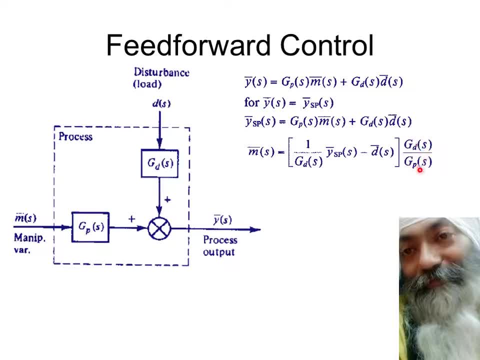 gc. gc means the uh you, you can say it's a transfer function of the controller- can be designed. the controller can be designed if we know the value of gd, if we know the value of gp, of course that will be called as gc. so we call this gc as the transfer function of the main controller, which 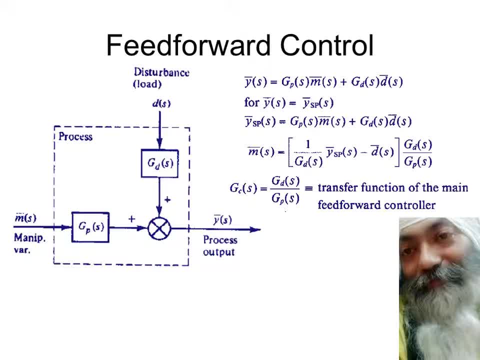 controller. mind you, it is a feed forward controller. that's equal to gd by gp. similarly, you can have another transfer function. we call it as gsp. that's nothing but one upon gd. it's one upon gd, as you can see over here. so let's try to uh give a graphical- uh- you can say uh- representation of this equation. 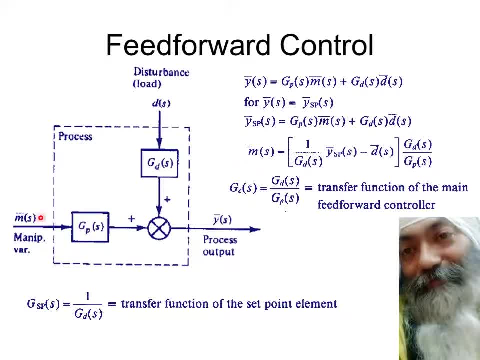 what is this equation? this equation is that this manipulated variable, this manipulated variable is equal to what i can just put one line over here. whatsoever is the change in set point. i will multiply by one, by gt. i will subtract the disturbance from here. i will multiply this by: 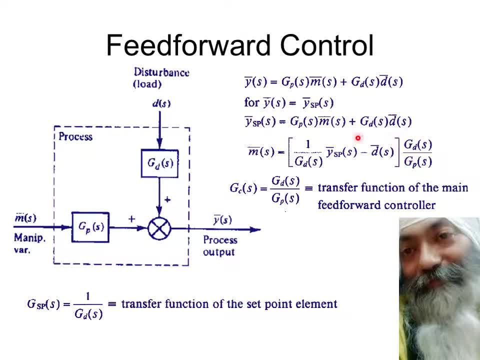 this vector gd by gp, and this entire signal will become ms manipulated variable and i'll put this over here. you can just imagine that i have some uh change in set point. that change in set point is multiplied by one upon gd. so i'll put one upon gd over here. i'll put a subtractor over here once i. 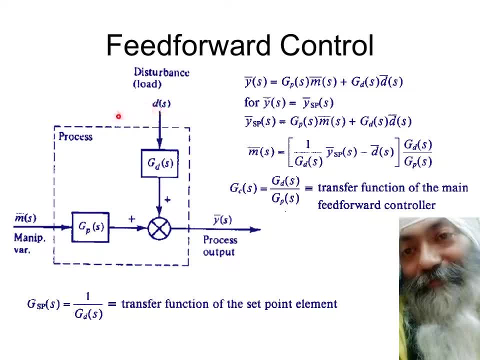 put a subtractor, this minus dc, this ds will be subtracted, and whatsoever is available over here is one upon gd into ysp minus ds. i'll multiply that by gd into divided by p. so this is multiplied by some gc, gc is nothing but gd upon gp, and that final thing, the output of that, is going to become. 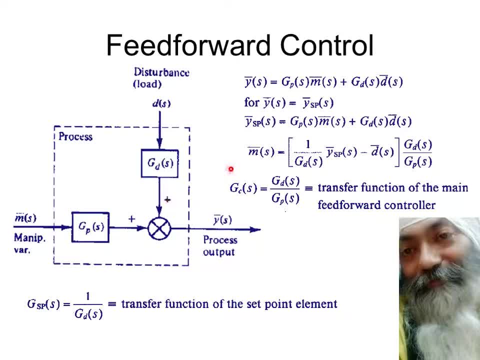 the input to this, that will become equal to the manipulated variable as given by this equation. so what we have to see is that i have gc given by this transfer function and i have gsp given by this transfer function. this is what i'm going to see in the next slide. 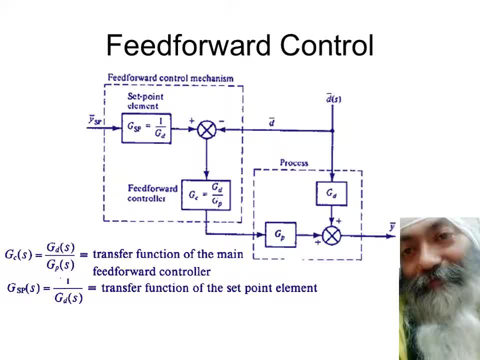 how do you friends? once again, as i said, this is gc given by gd upon gp and this is gsp given by one upon gd. this is what i told you, that you have some transfer function, uh, of the change in set point, it's going to be multiplied by one upon gd. so this: 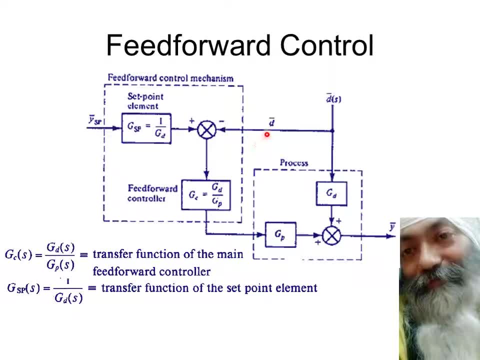 ysp will get multiplied by one upon gd and this d will be subtracted from here. you will get over. here is ysp upon gd minus t. this will get multiplied by gd upon gp and this final thing will become equal to the manipulated variable which will go over here. and that is how the whole. 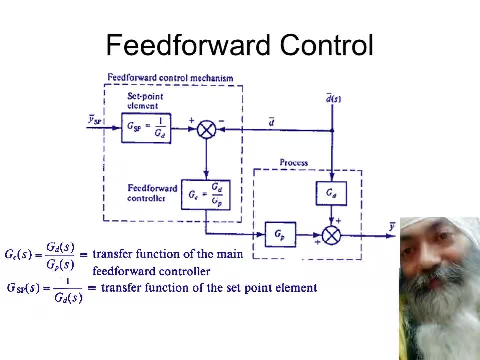 feed forward control loop. that is upon this philosophy to keep y bar constant. so the thing is that, as you can see in the last line, the forward control design of the forward control depends heavily on the good knowledge of process model gp upon gd we can design this feedback. 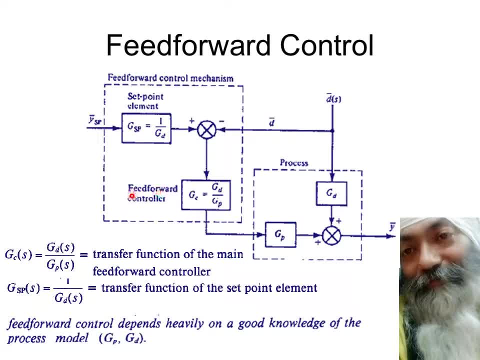 feed forward. i beg your pardon, it's feed forward controller. uh, in a manner only if this gd and gp are properly known to us. if this gd and gp are not known, then this gc can never be designed. apart from that, we also have a condition that we might be knowing gd, we might be knowing gp, but we have to make sure that this gd upon gp 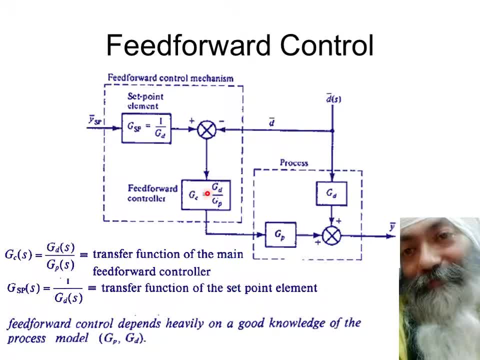 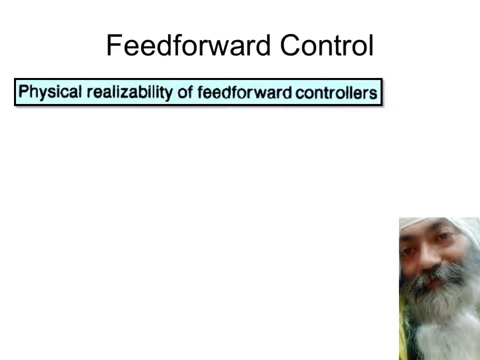 ratio. it has to be physically realizable. it has to be physically realizable. what do you mean by physically realizable? that also we will see subsequently. so physical reliability of the feedback- i beg your pardon once again, because so used to saying feedback it's actually feed forward. so if the physical reliability of feed forward controllers 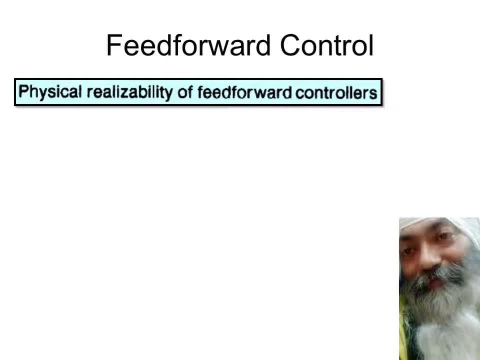 uh is is explained with help of an example that, let us say, dp is given by some term into ed power minus 0.5, gd is again some term into ed power minus 0.1. you know, here the delay is more in case of process and 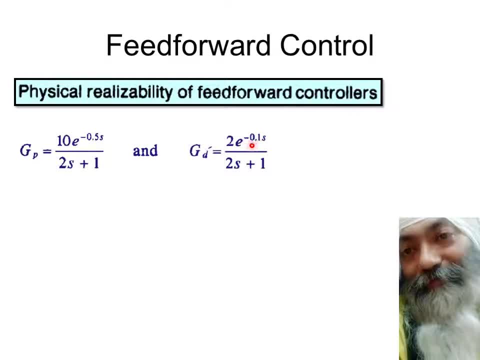 the disturbance is acting later and the delay is slightly less. it is 0.5 second delay. it is only 0.1 second delay. so in this case, if you will try to make the c and gc is nothing but gd upon gp and as you divide you will have the final transfer element, the final uh transfer function and the 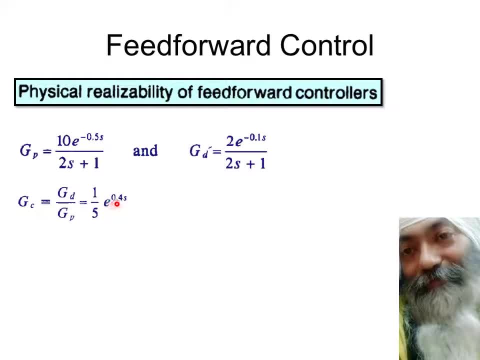 that comes out to be e, the power plus 0.4 plus 0.4. this is the delay element. that is, we know the element is getting delayed. this is something which is opposite of delay means we need the future value. no system as such can predict the future value of any signal and therefore these: 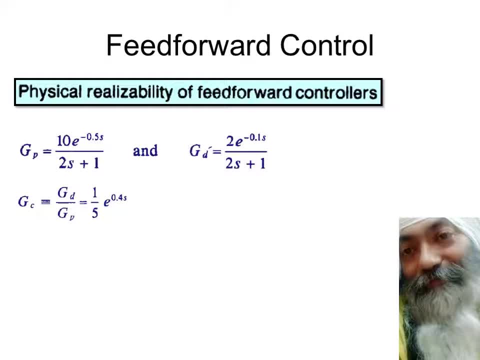 kind of controllers are not physically irrealizable. they are not physically illausible. so these kind of feed forward controllers are not physically irrealizable. so the exponential term requires future values, that is, it requires the value of disturbance to be known in future. not the current value but the future value of disturbance is required to compute. 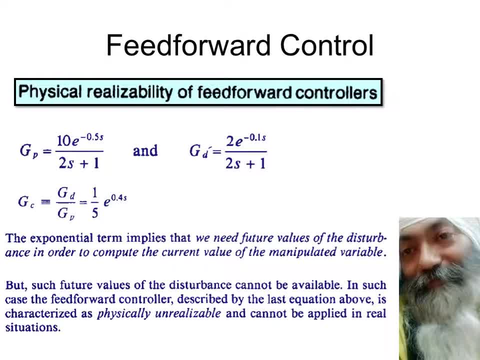 the current value of disturbance value of manipulated variable, which is not possible. so that's why we say, because the feature values are not known to us, these kind of feed forward controllers, especially here, as you can see in these examples, as we can see over here, are physically unrealizable, they cannot be applied in the real situations. 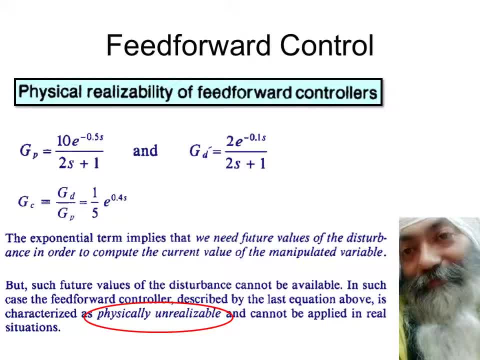 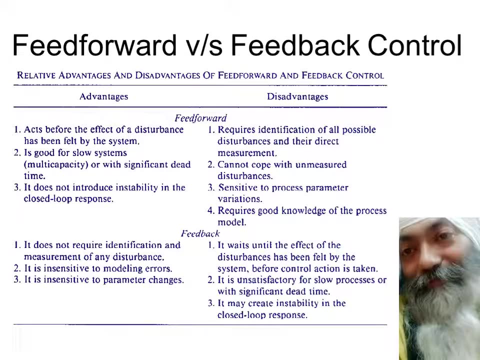 you just cannot simply know that. I know the mathematical model and I will design it. it's not possible. only if it is physically realizable we can go in for these kind of controllers. otherwise, not coming to both the traditional feedback controller and the feed forward controllers as we have studied over here, you have the advantages and disadvantages. 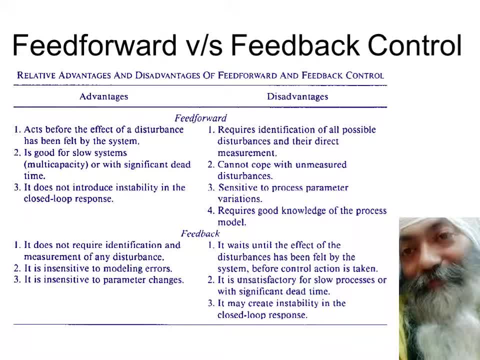 of both feed forward and advantages and disadvantages of both feedback controllers as well. and feed forward you have learned today and the feedback you already know. they are being summed up in this table over here. first, we will consider the advantages of feed forward controller. the first one, as you can see, is that it 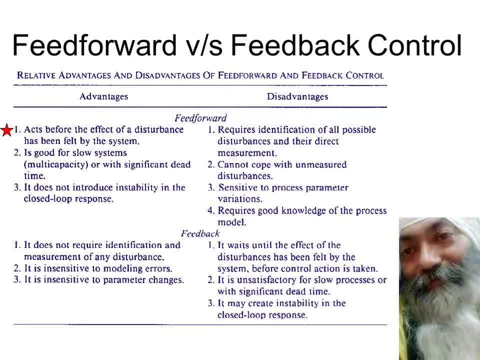 acts, for the effect of disturbance has been felt by the system. it's good for slow systems with significant dead time, for example. it does not introduce stability. this is the part of feed forward. control will never, ever result in instability, which is not possible in the real world. so this is the first one. 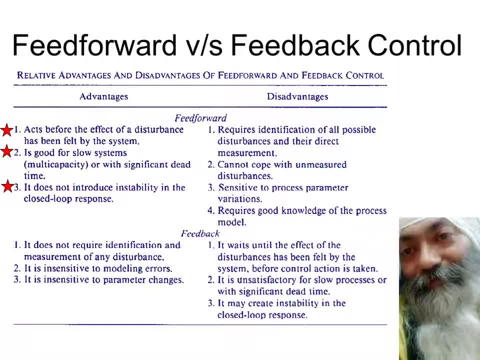 which is quite common in case of feedback controls. we are. if you increase the gain, then with higher gain the feedback control system tends to become oscillatory. feed-forward control will never become oscillatory, but then you have disadvantages of feed forward. number one: it requires the identification of all possible disturbances and their direct 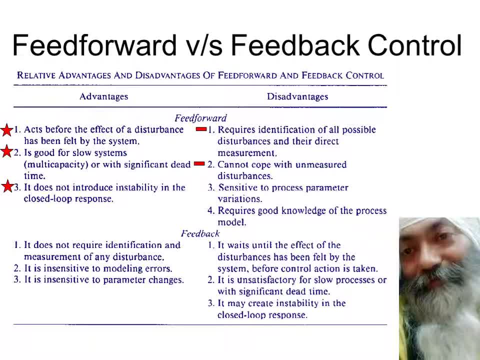 measurement, so the disturbances have to be measurable. it cannot cope with the measurements which are not measurable. it is sensitive to the process parameter variations, because we need to know GP and GD. it requires good knowledge of the process model as such. so these are the advantages and disadvantages of 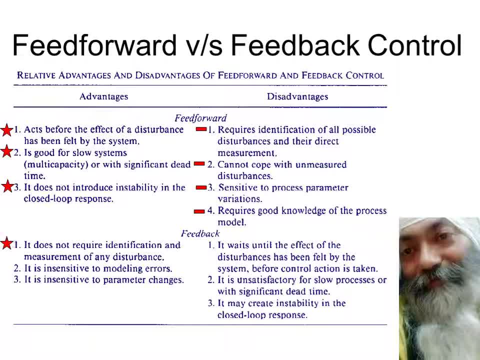 feedforward controller compared with that of the feedback controller, which does not require any kind of measurement of disturbance. it is insensitive to the relatively quite insensitive to the modeling errors and it is insensitive to the parameter changes that may be taking place in the model. but then again, 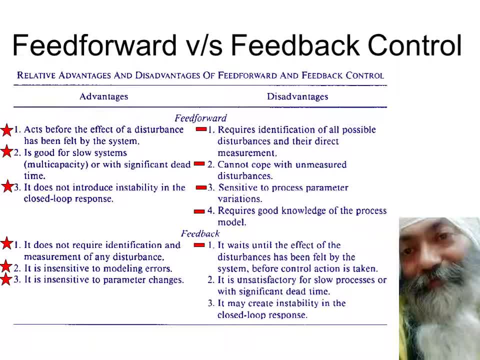 it has some disadvantages also. first of all, in case, the biggest disadvantage of feedback is that it waits. it waits until the effect of disturbance has been felt. so it's a damage control. some damage is happening, and then it starts to control it, but it's not taking action before the damage. the second thing is: 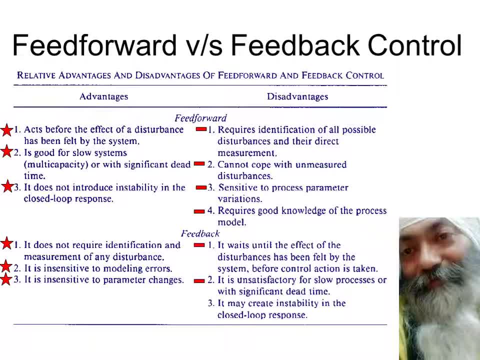 that it is unsatisfactory for the slow processes with the significant loss of time, dead time and many times if we are not giving a proper gain, we give slightly more gain to the feed back system. they may create instability in the closed loop, so the system tends to become unstable and oscillatory. so what we do? 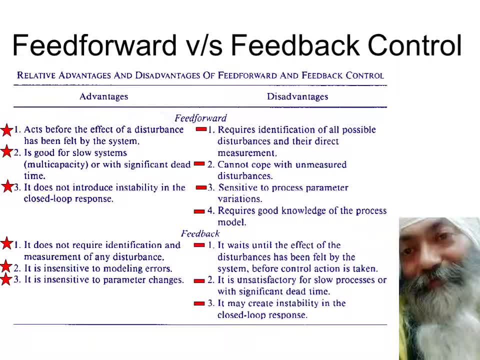 is that to take the advantage of both feedforward and feedback systems. we combine the two. we make use of feedback and feedback. in aуль we make use of feed forward primarily every making you the feed forward. we trying to mitigate most of the disturbance effects by feed. 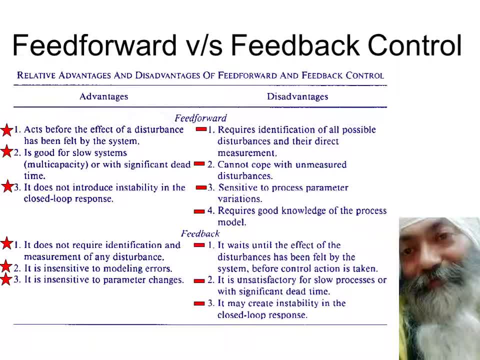 forward. but because of the unknown values of the parameters and so on and so forth, some of the disturbances may not be so accurately measured, and so on and so forth, the feed forward control is not able to fully compensate for the disturbances. so the remaining parts, part of it, say thirty percent. twenty percent of it is still not fixed. so it is vanishing. this will come closer to the end of today's session. I will get into this next slide and then go into more detail soon, but let's just complete this chapter. we will be finishing this part after two hours. this is the next part. then this is the comminium part of the by-products. now the power Mickophone. 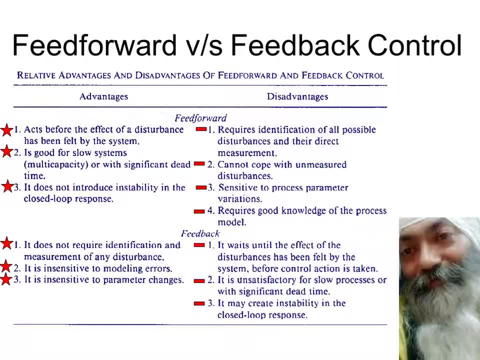 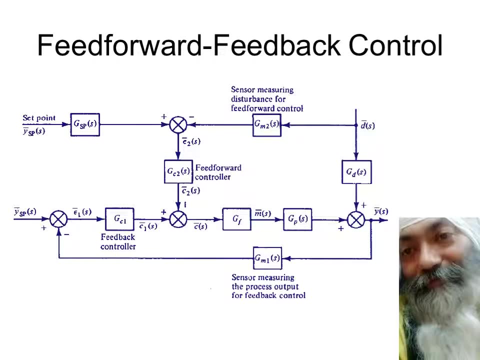 it is compensated by a feedback. so we use both feed forward as well as feedback control, especially the critical, very, very critical uh situations. that's what we're going to see in the next. so here you see, in the next, in this slide, you have a feed forward as well as a feedback controller. 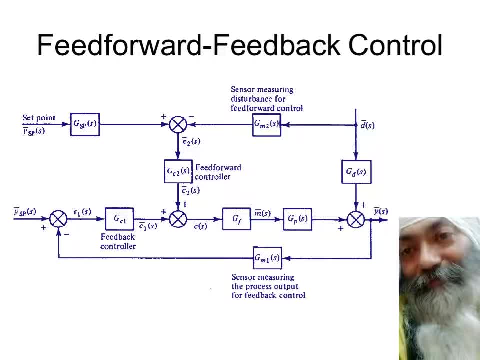 first of all, you see that it it has a traditional feedback control. as you can see, over here you are taking the feedback, uh, and along with it you have a feed forward controller. as you can see from here on the top, the top most one is having feed forward, the lower one is feed back, that's. 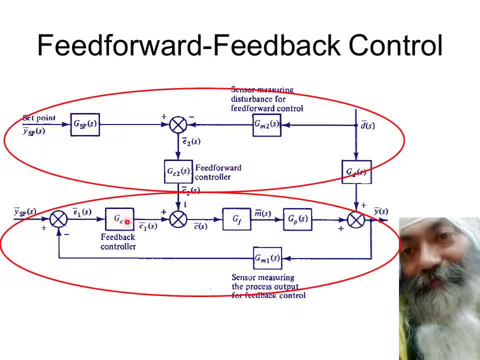 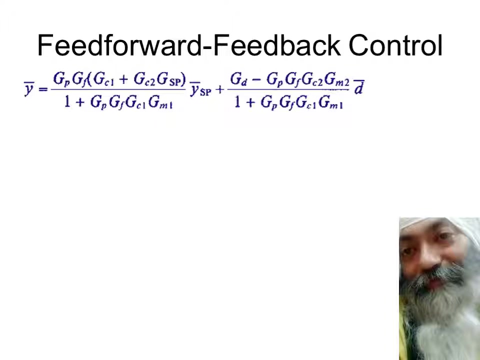 how you controller used, given the thing c1, and for the feed forward, the controller is given the notation of gc2. that is, what we do is that we analyze this and we will get a mathematical equation as for the output given in the next slide. so what you see over here is the output given by both feed forward and 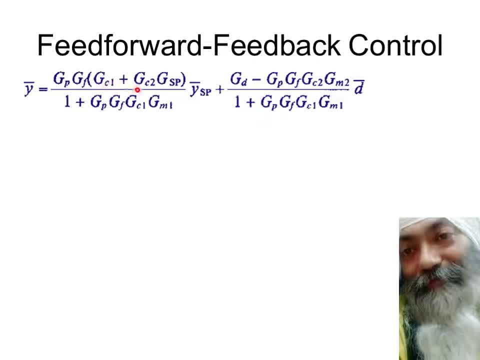 feed back. c1 is for feedback, c2 is for feed forward. but the interesting thing is that if you see the denominator denominator has only gc1 denominator has only gc1 denominator. gc2 is missing. gc2 is for feed forward, gc1 is for feedback. so it means that the denominator, the one which is going to determine, 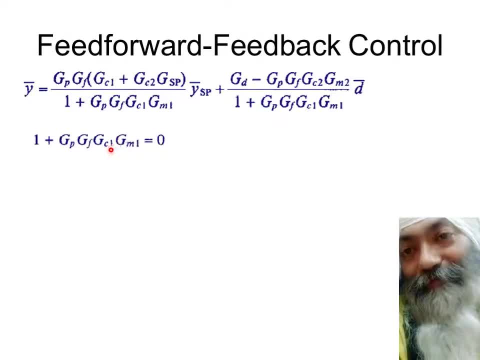 the stability and the characteristic equation is dependent only on the feed back controller. feed forward will never, ever make the system unstable. unstability or instability in the system will be introduced, if at all, only on account of the feed back controller. so we have gains of feedback quite low, so as to not get into an oscillatory behavior or things becoming unstable.